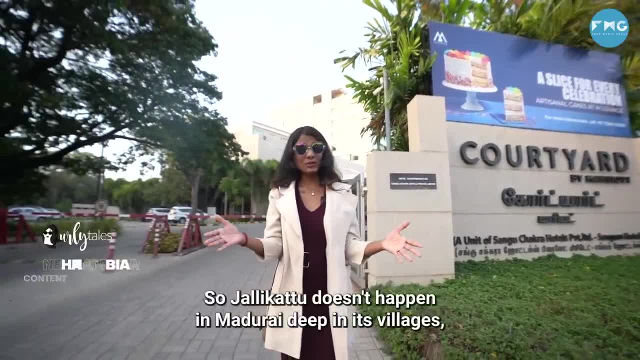 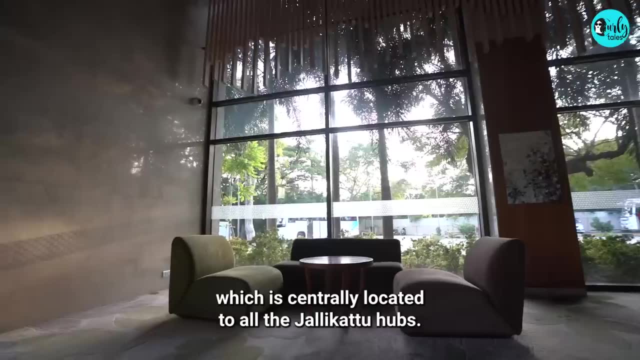 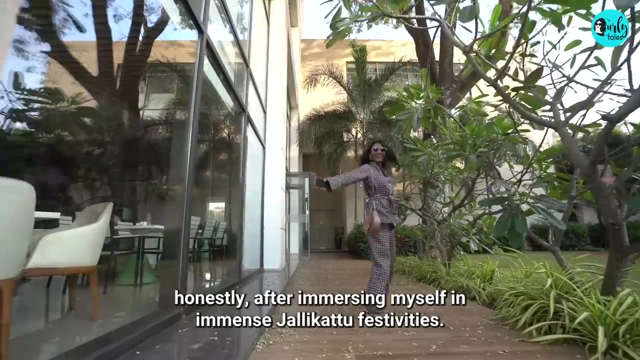 So Jallikattu doesn't happen in Madurai, but deep in its villages, Which is why I'm staying at Kotyad Marriott in Madurai, which is centrally located to all the Jallikattu hubs. It's comfortable, elegant and the perfect place to crash honestly after immersing myself in the immense Jallikattu festivities. 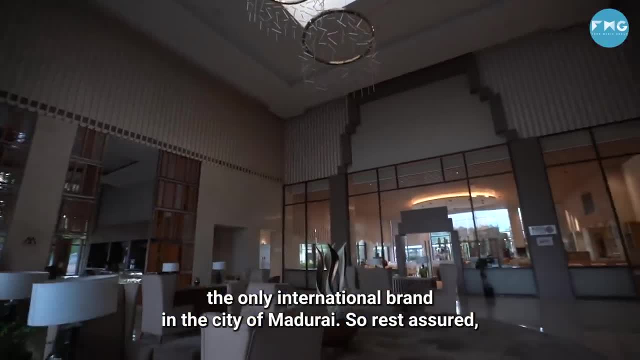 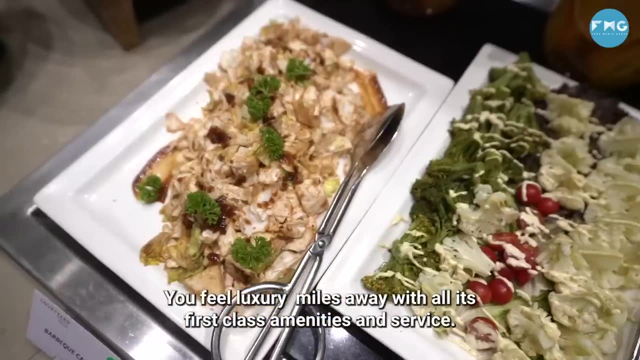 Kotyad Marriott also happens to be the only international brand in the city of Madurai, So rest assured you feel luxury miles away, With all its first-class amenities and service. My favourite of all was the Madurai Thali. They're truly experts in luxury. 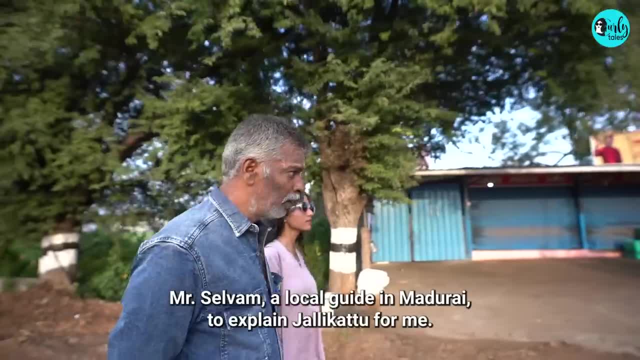 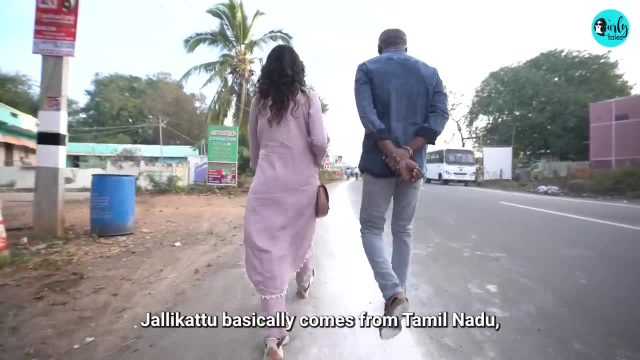 And speaking of experts, I met with Mr Selvam, a local guide in Madurai, to explain Jallikattu for me. Jallikattu basically comes from Tamil Nadu. That's a traditional sport from the beginning. 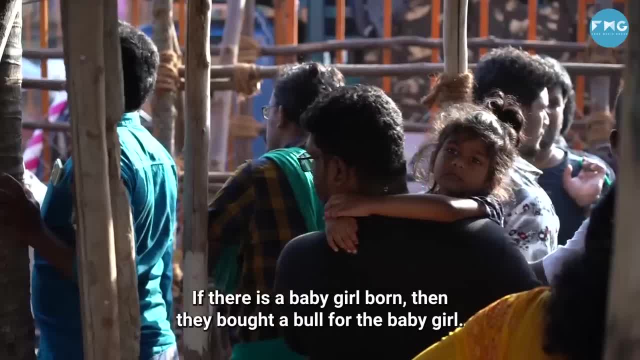 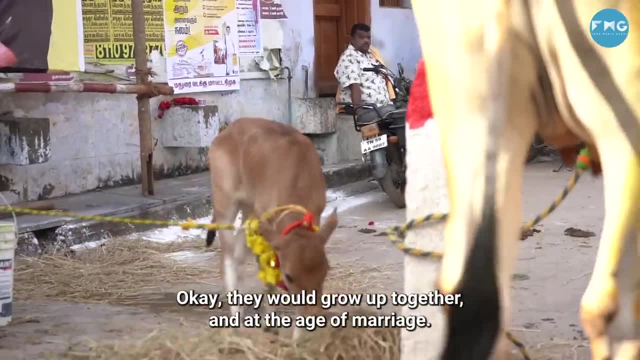 In the olden days, for an example, if there is a Jallikattu festival, the baby girl is born, then they bring a bull for the baby girl. They grow up at the same periods, same levels. At the age of marriage they do the sport for the girl. 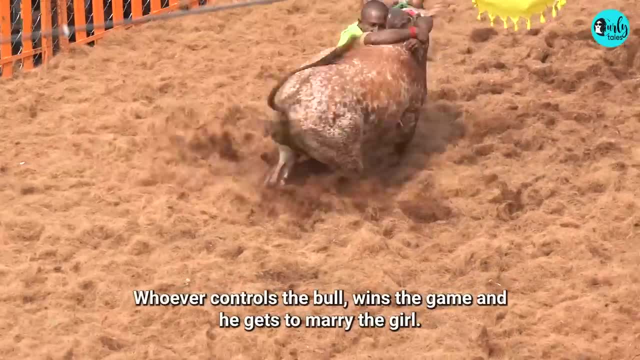 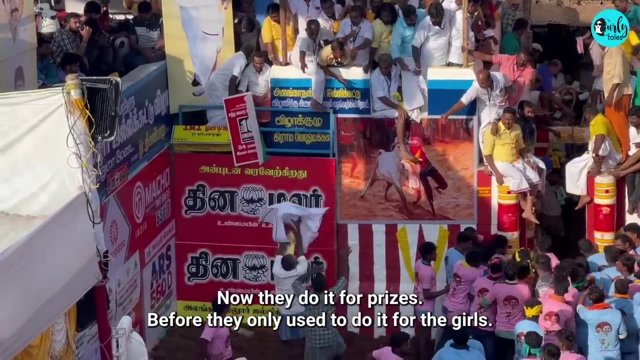 Whoever controls the bull, they are the winners. They marry the girl. That's how it starts the Jallikattu Now. they do it for prices Before. they only do it for the girls. People say that this is cruelty. 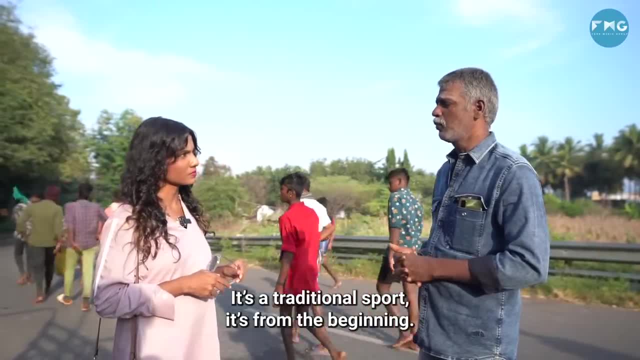 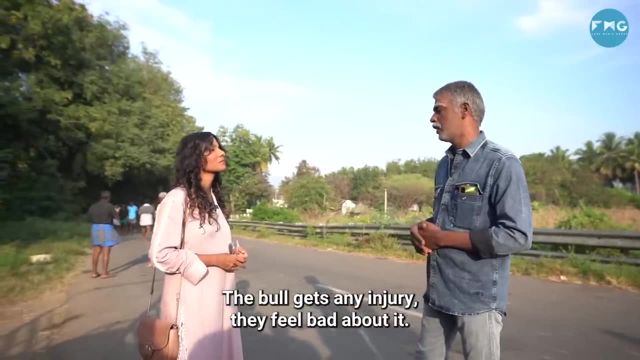 There is no cruelty. That's a traditional sport. It's from the beginning. If you go to their houses, they treat them like a baby. If the bull gets injured, they feel very bad about it. That's a bad sign for the family. 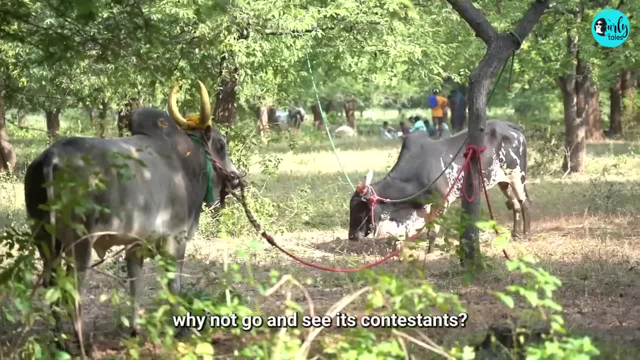 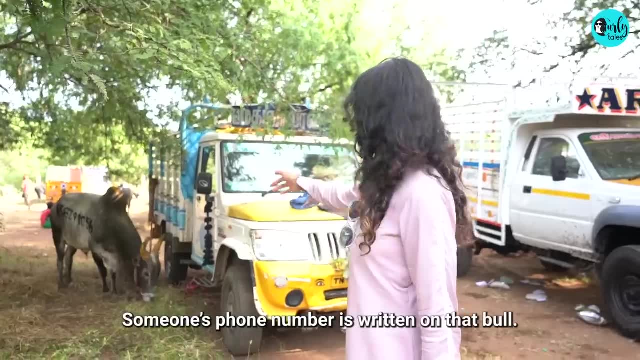 Now, before watching the game, I thought why not go and see its contestants? So I walked towards a shed where the bulls and bull owners were waiting for their turn. Someone's number is written on top of a bull Writing numbers on bulls in case they got lost. 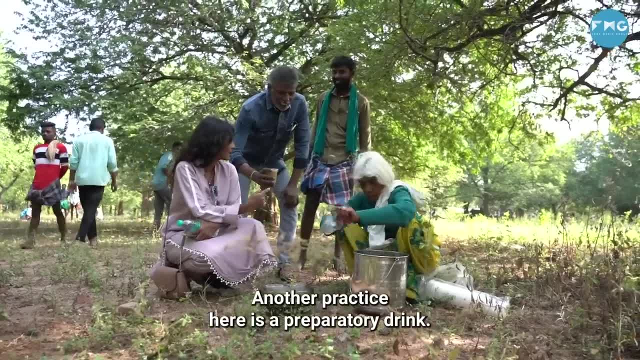 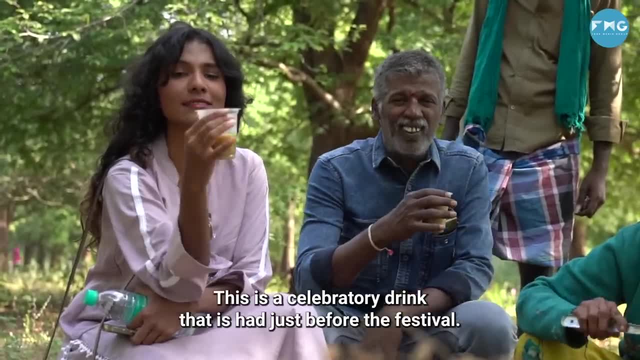 is very casual here. Another practice here is a preparatory drink. Oh, cotton seeds. Okay, okay, okay. Parthipal is made of cotton seeds and milk, And this is a celebratory drink that is had just before the festival. 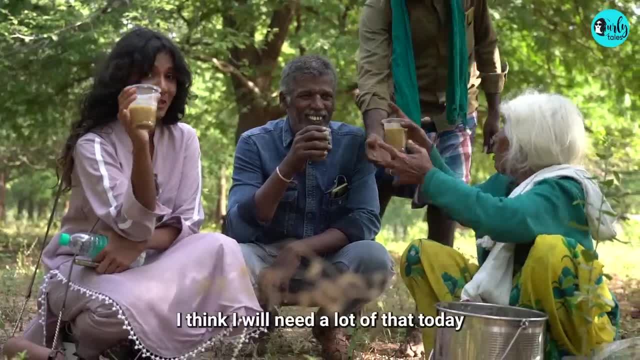 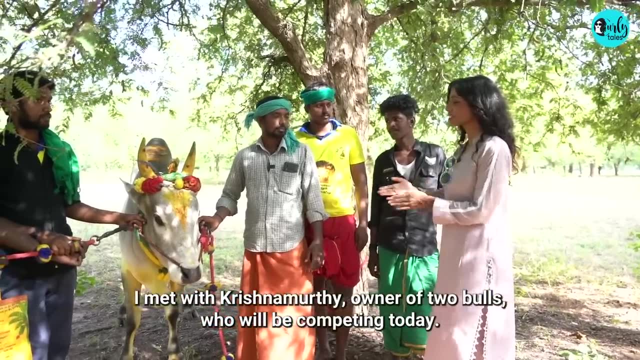 Energy drink, Energy drink. I think I'll need a lot of that. today. I met with Krishnamurthy, owner of two bulls who will be competing today. Are you nervous about your bull taking him to the field And do you feel scared if anything happens? 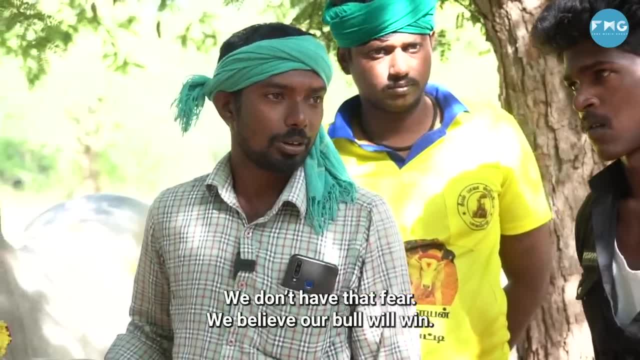 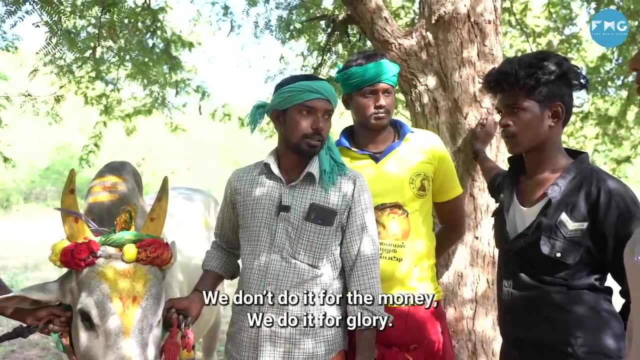 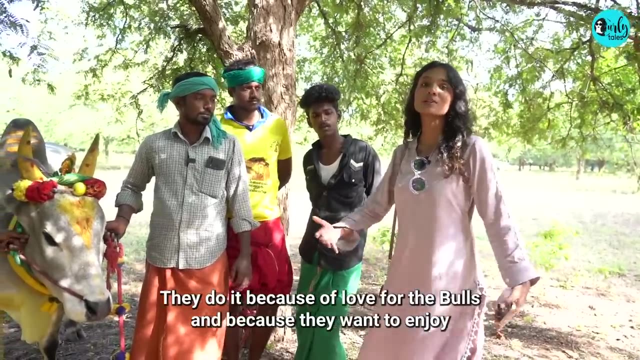 Nothing happens to him. There is no such thing. Our bull will win. We have that belief. Our bull will win. It's not for money, It's for fame. So basically, they don't do it for winning the money. They do it because of love for their bulls and because they want to enjoy and play the sport. 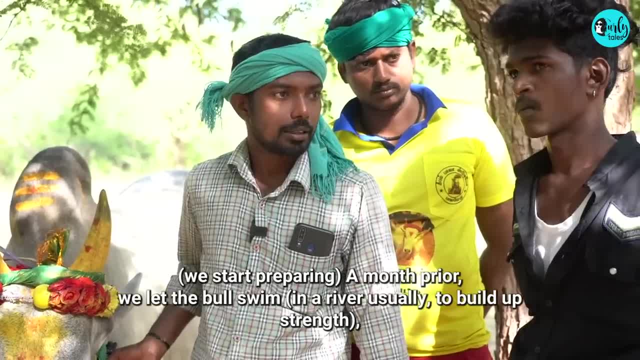 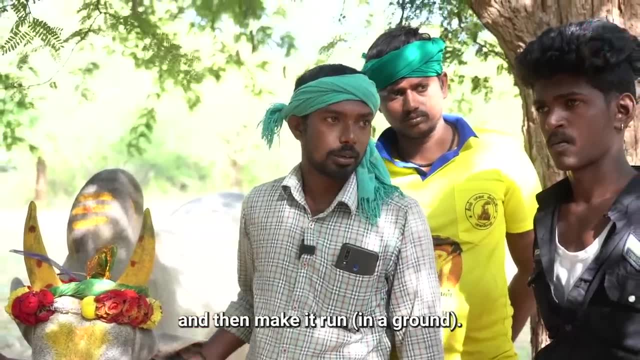 How did you prepare this bull? A month ago, I prepared a bull like Neechal, Karthiyotha and Nadabudikirathu. After that, I brought it to Jallianth Wow. Out of 37 indigenous cattle breeds in India, a large number come from Tamil Nadu. 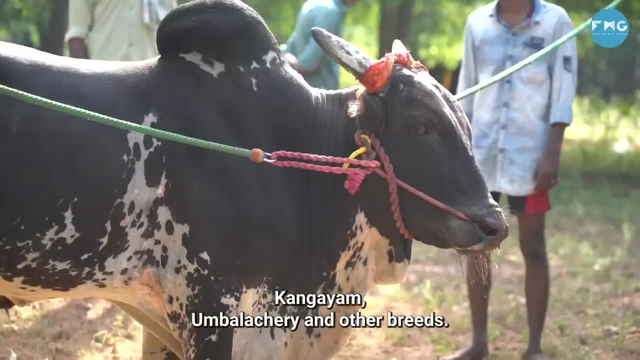 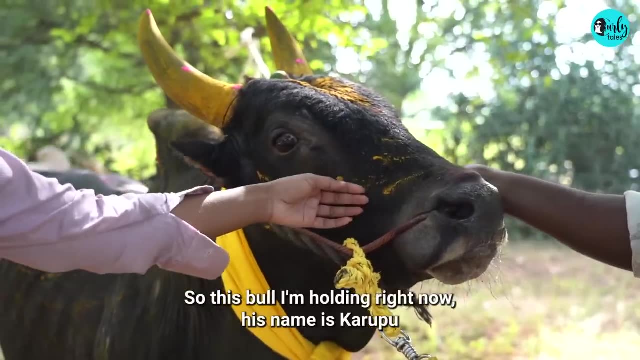 These include Pulikulam, Kangayam, Oombala, Sherry and other breeds, And for this sport the bulls mostly used are Pulikulam. So this bull I'm holding right now, his name is Karuppu. 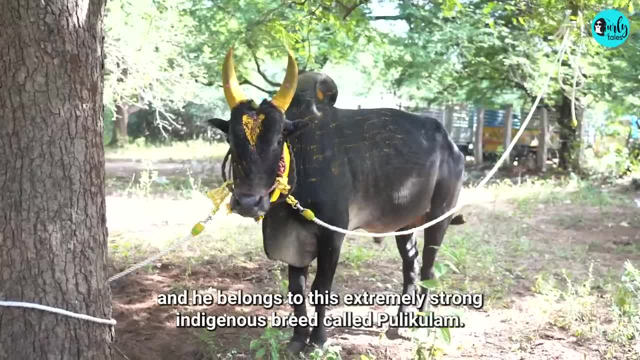 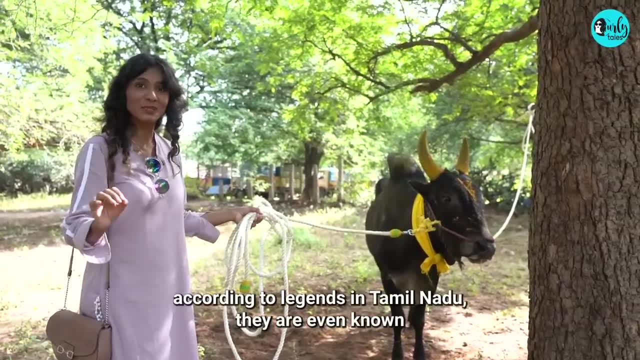 And he belongs to this extremely strong indigenous breed called Pulikulam. Pulikulams are very hefty, strong and, most importantly, according to legends in Tamil Nadu, they are even known to drive away tigers from villages. That's how strong they are. 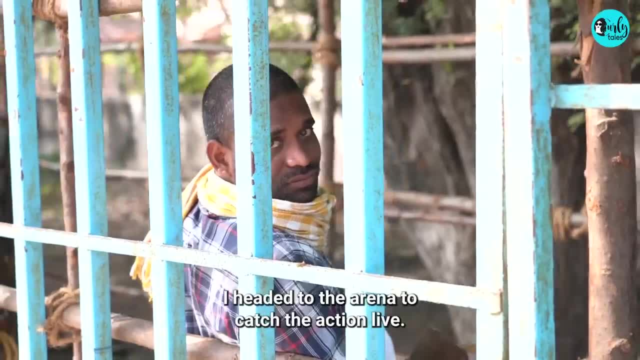 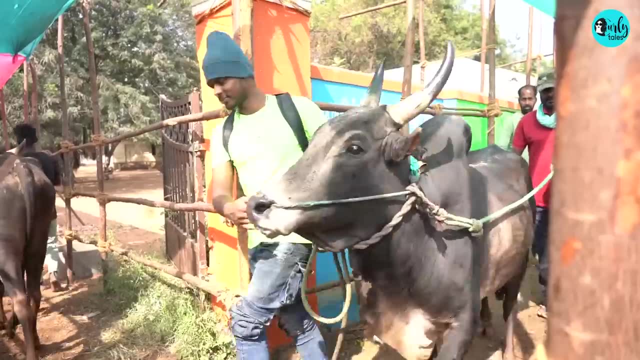 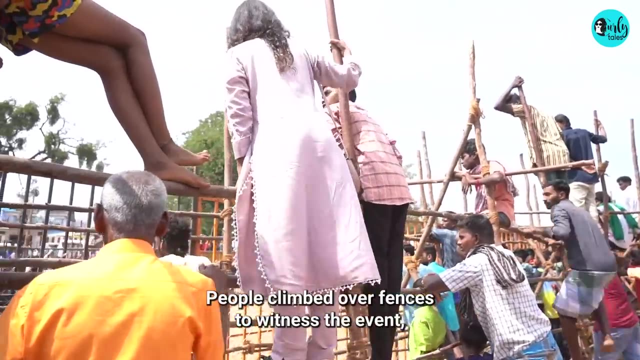 Now, while the bulls and bull tamers prep for the competition, I headed to the arena to catch the action live. The arena of Palo Medo was electric. People climbed over fences to witness the event, With police standing near the barricades to prevent any casualties from happening. 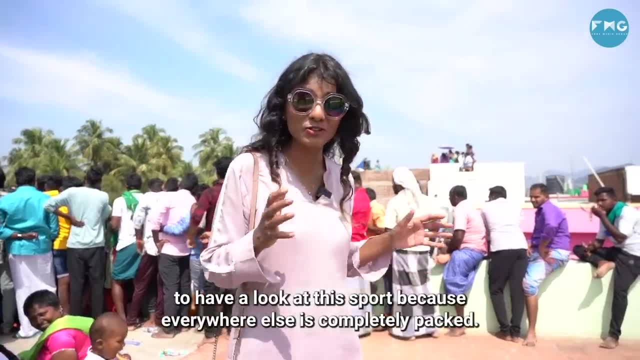 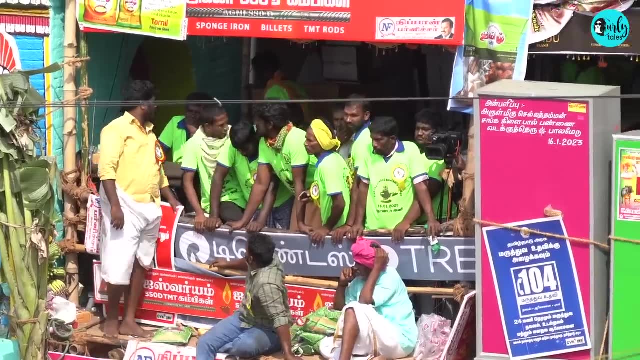 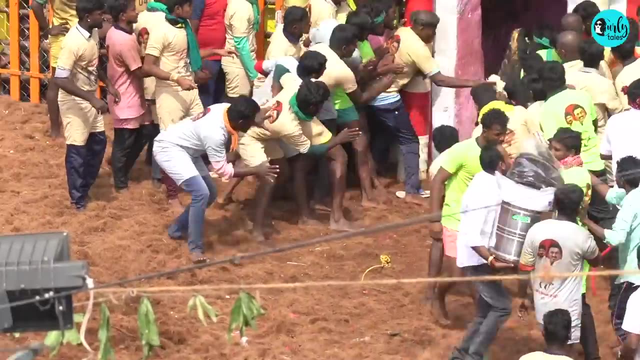 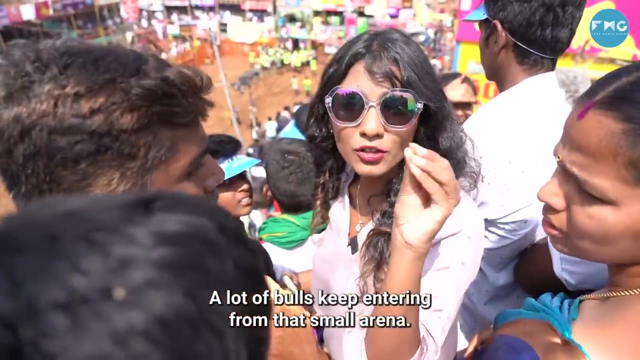 I'm actually at a complete stranger's terrace to have a look at this sport, Because everywhere else is completely packed. That's how crazy people are about this festival. So from what I can see is happening here, a lot of bulls keep entering from that small arena. 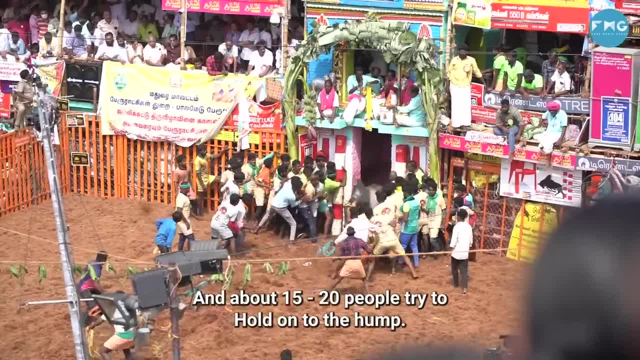 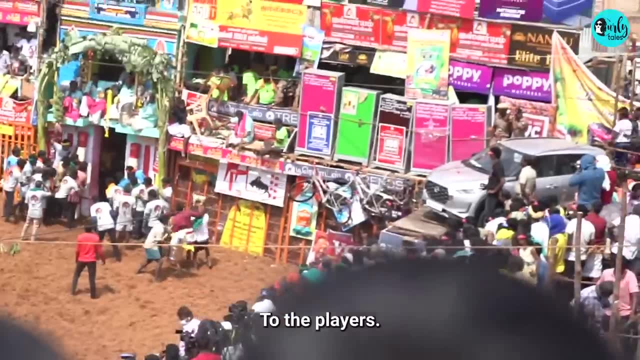 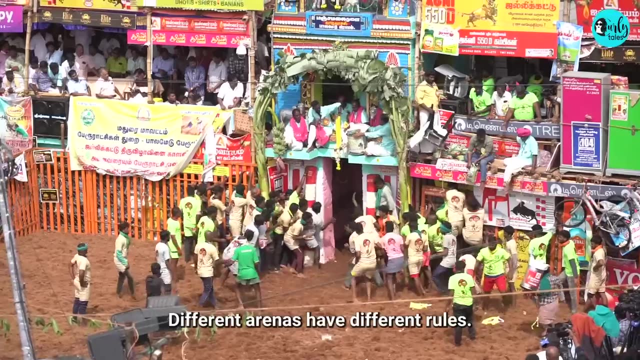 And about 15-20 people try to hold onto the hump. They have a duration of about 15-20 seconds to do that And if they do that they get prizes thrown from the top to the players. Different arenas have different rules. 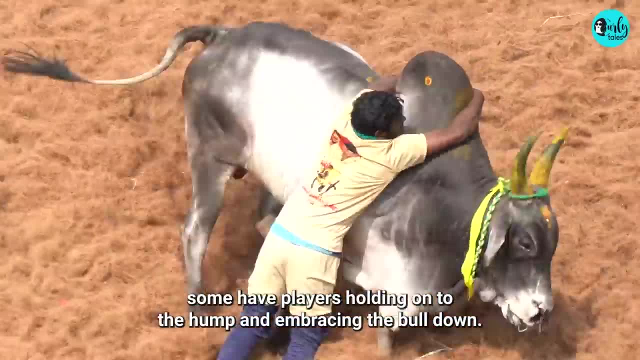 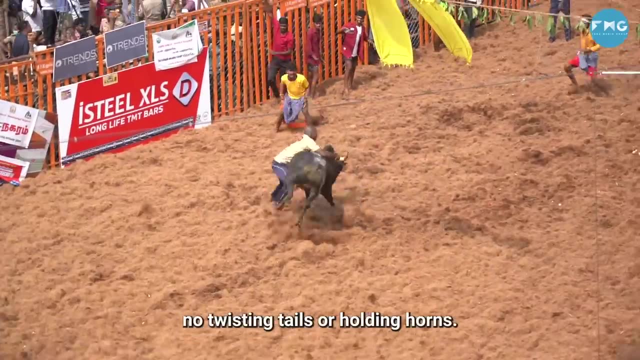 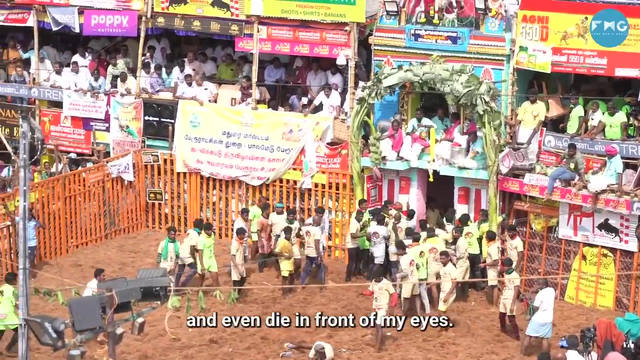 Some have coins attached to the horns, Players holding on the hump and embracing the bull down. However, general rule of thumb is that two people cannot hold onto the hump at one time, No twisting tails or holding horns. This is the most difficult thing I've had to watch to see people get injured and even die in front of my eyes. 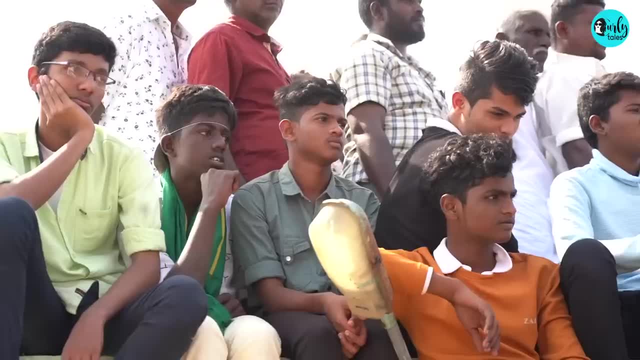 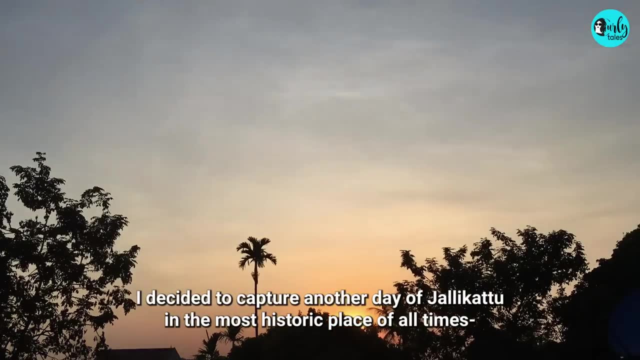 It's too much. I wonder what their families might be going through. After a difficult first day of witnessing people cheering for their bulls and bull tamers, I decided to capture another day of Jallikattu in the most historic place of all times. 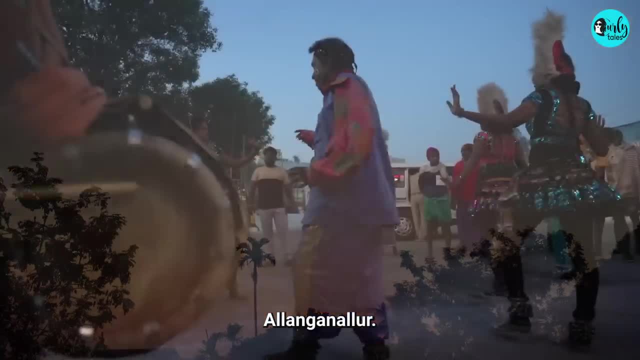 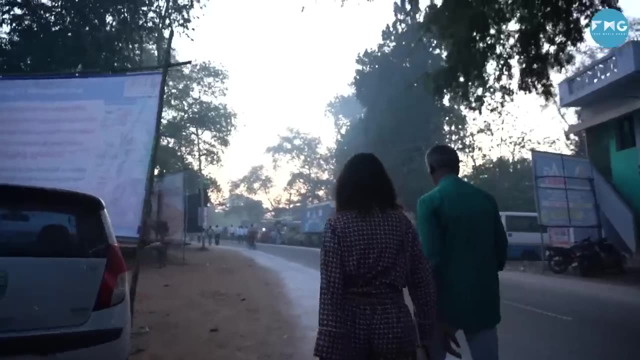 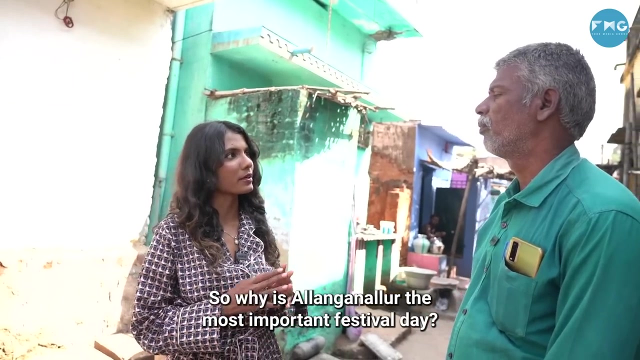 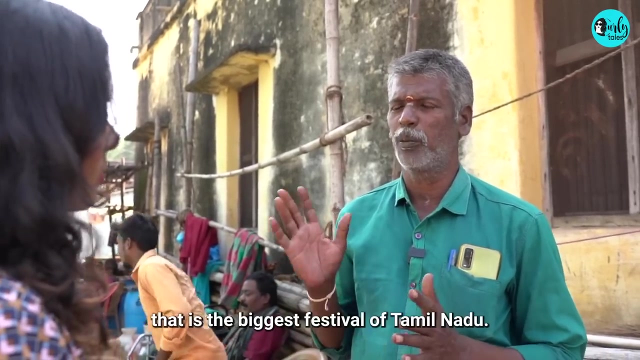 Alanganallur. So why is Alanganallur the most important festival day? They bring a statue of Vishnu. while they celebrate the Chitre festival, That is the biggest festival of Tamil Nadu, They bring a statue to cross over this festival. 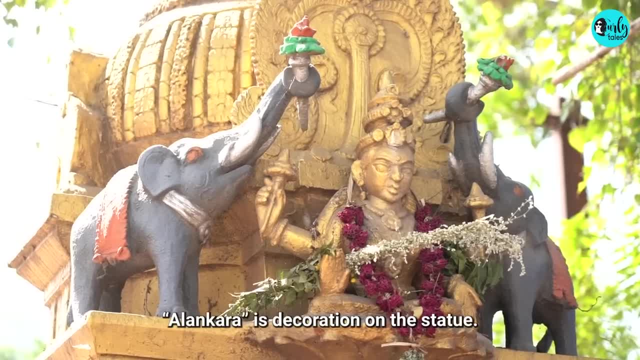 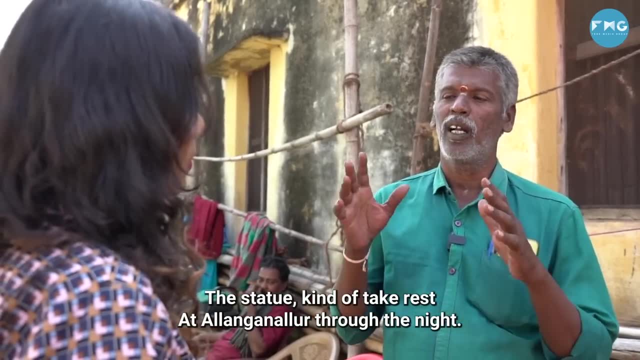 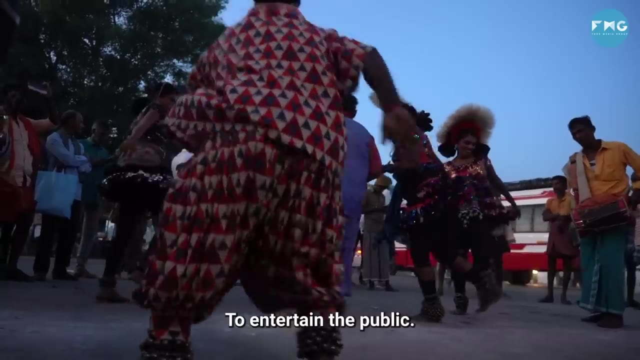 The village. the time they put down here they do some Alangar. Alangar means decoration of the statue. The statue they take rest, kind of rest, they do at Alanganallur for the night. That time they do this celebration, the festival, Jallikattu festival, to entertain the public. 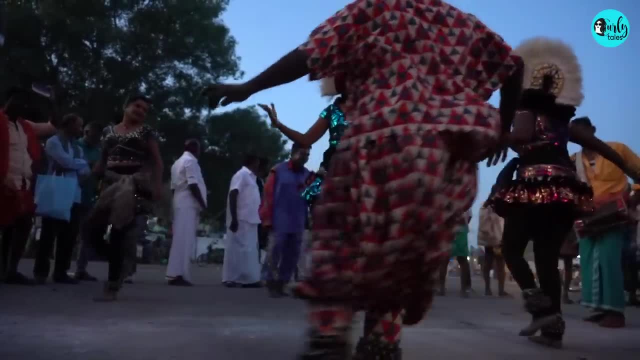 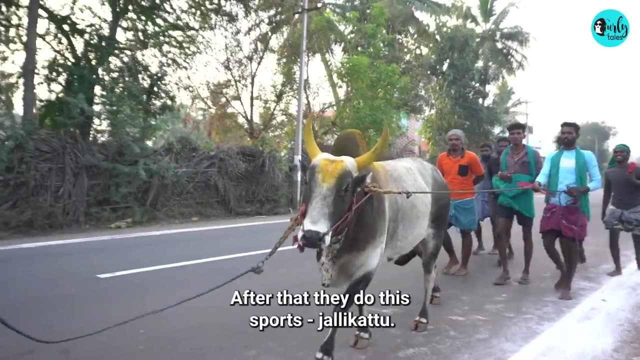 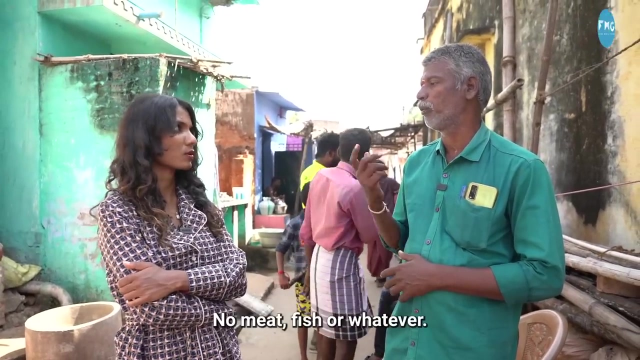 That's why it's very famous. It's accompanied with mythology. They celebrate the harvesting festival. So the farmer, they work continuously for five months to take the harvest. After that they do this sports- Jallikattu. Before that they do not take any non-vegetarian, like meat, fish, whatever they want. 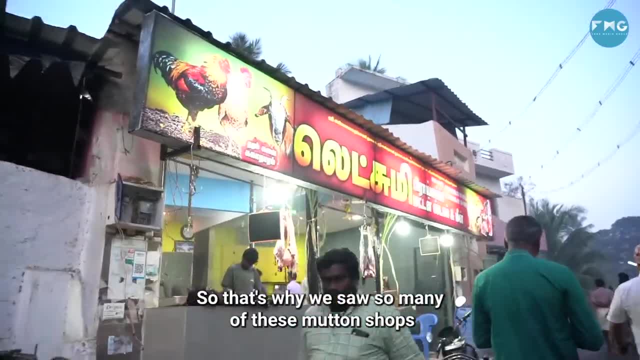 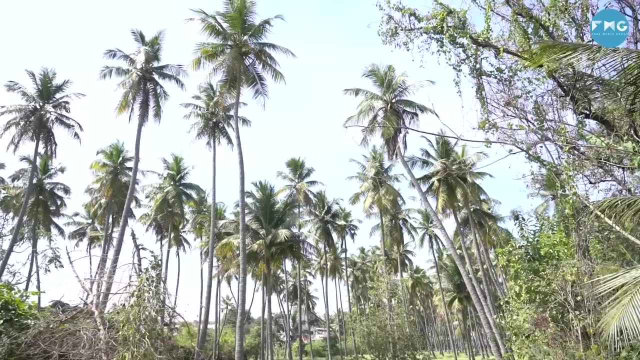 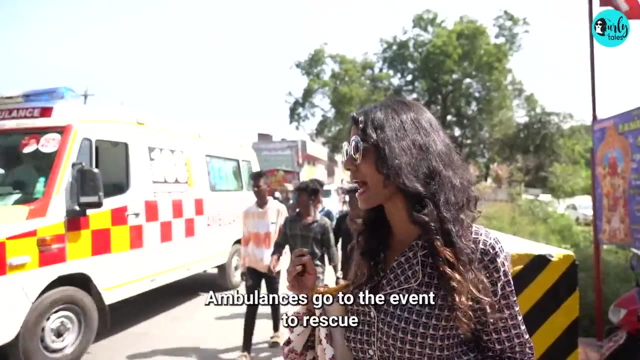 So that's why we saw so many of these mutton shops- Yeah, mutton shops. That's why you saw that they got the goat on the way. Ah right, Okay, Ambulance is here Because there are so many multiple injuries on sport. ambulances go to the event to rescue such injuries. 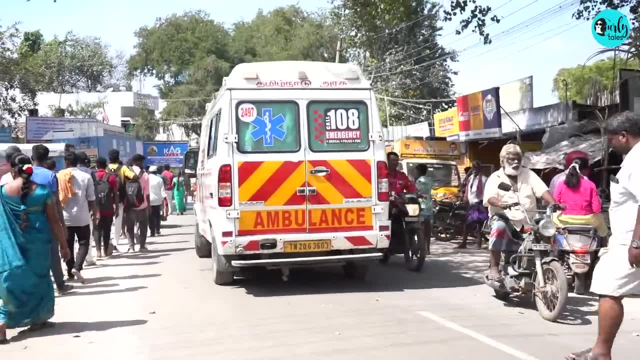 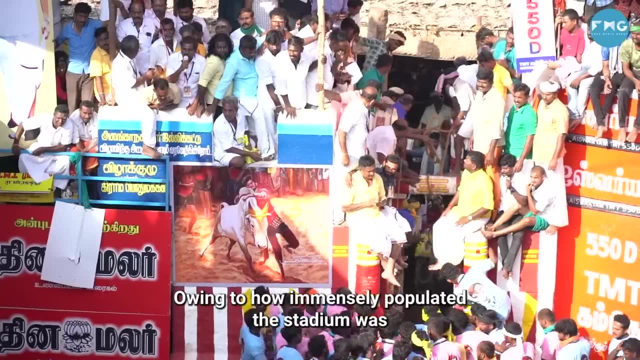 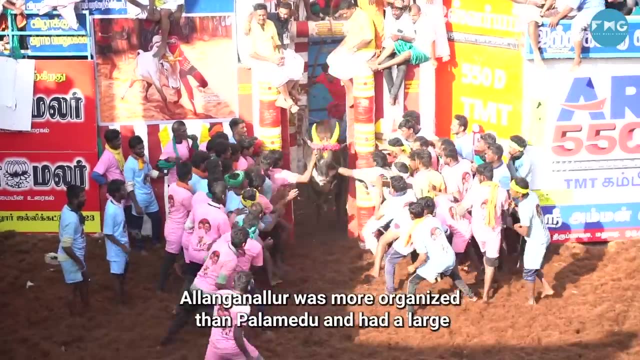 And they are injured players. Owing to how immensely populated the stadium was, I ended up on a stranger's terrace to witness the sport. Alanganallur was more organized than Palamedu and had a large number of bulls running in, as this was also the last day of the festival. 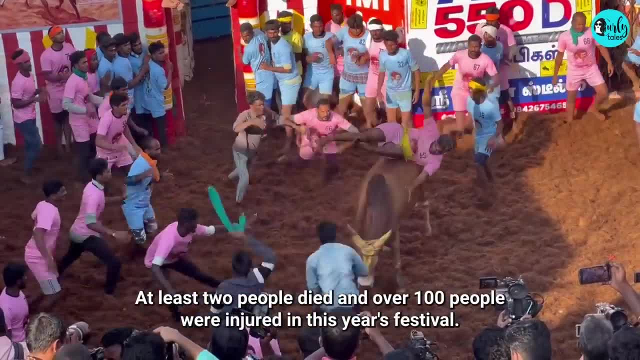 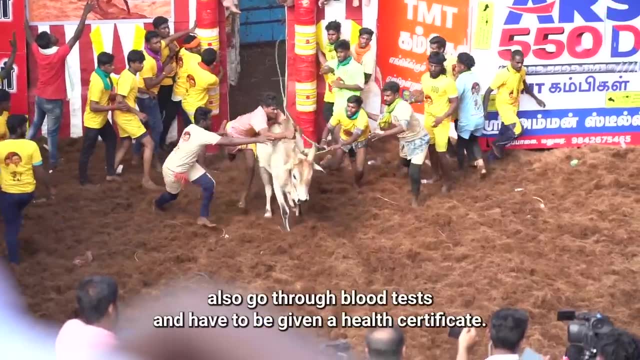 At least two people died. Several people were injured in this year's festival. Ambulances and other facilities were kept as close to the site for any mishaps. In addition to that, bulls also go through blood tests and have to be given a health certificate. 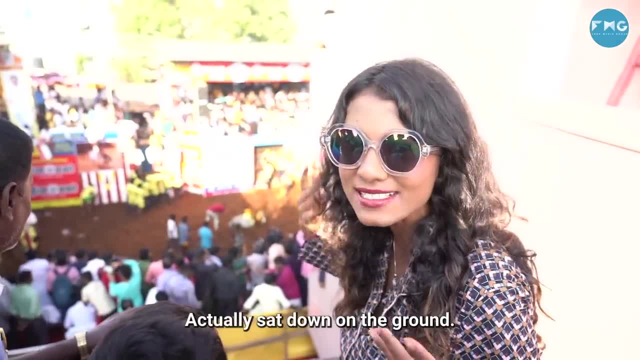 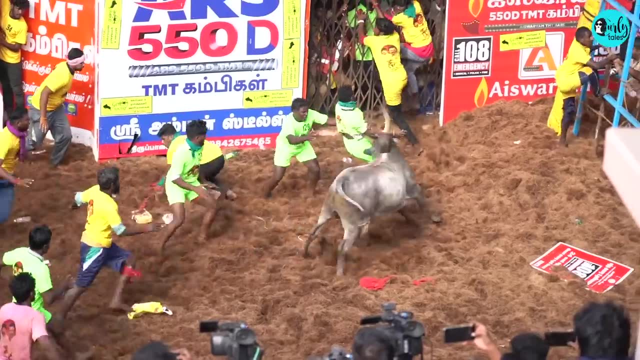 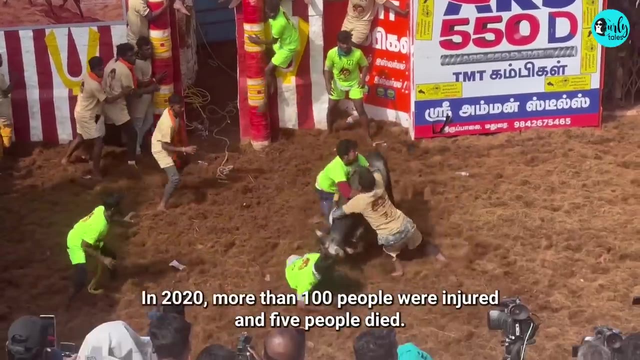 The bull who was supposed to be charging on people actually sat down on the ground. Oh my God. Despite precautions, many people and animals continue to die and get seriously injured playing this sport. In 2020, more than 100 people were injured and 5 people died. 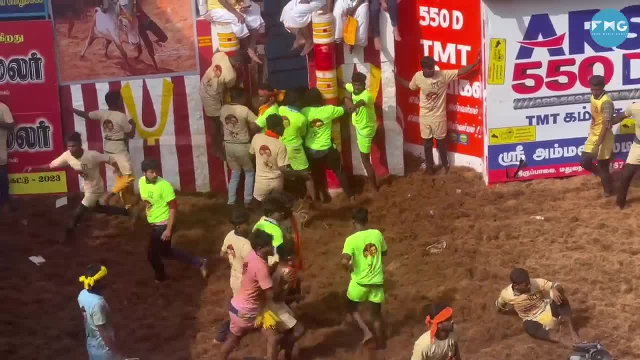 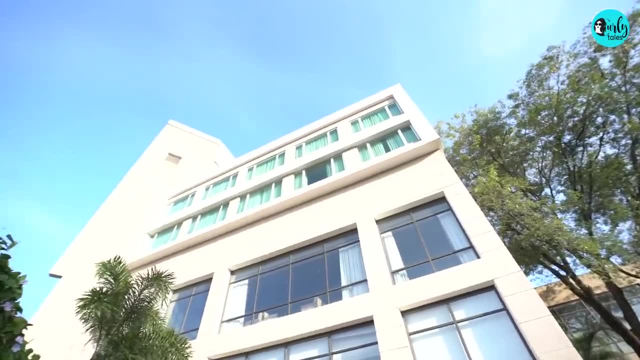 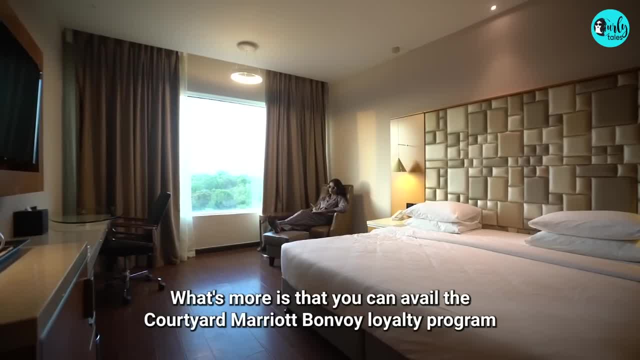 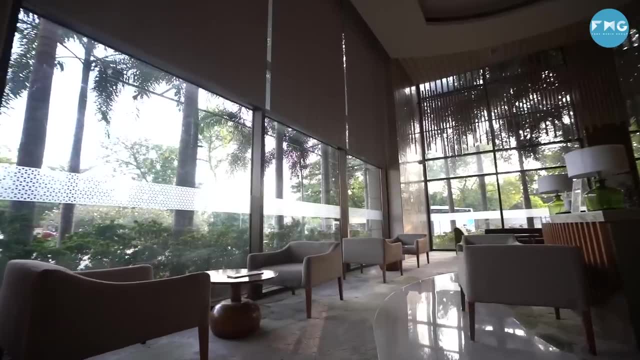 organising such a comfortable and cosy stay here. What's more is that you can avail the Kotyad Marriott Bonvoy Loyalty Programme, wherein the more you stay with Kotyad, the more perks you avail, such as perks on flights travel. 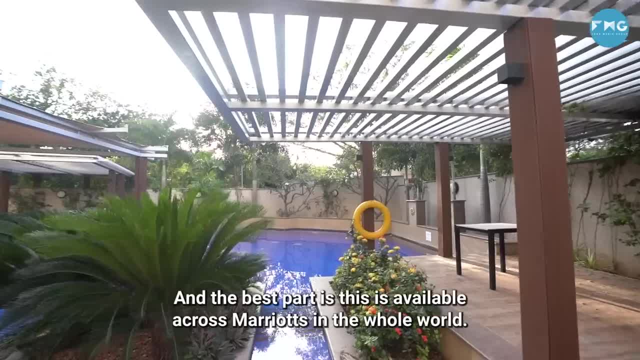 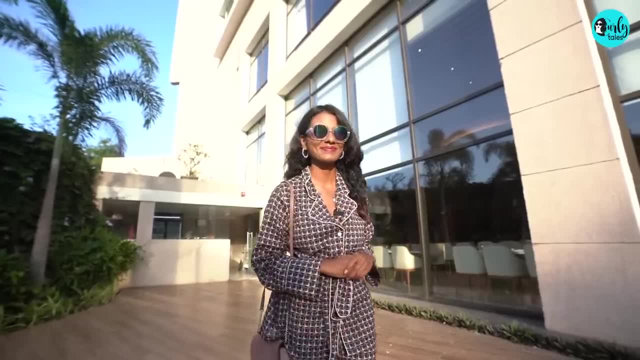 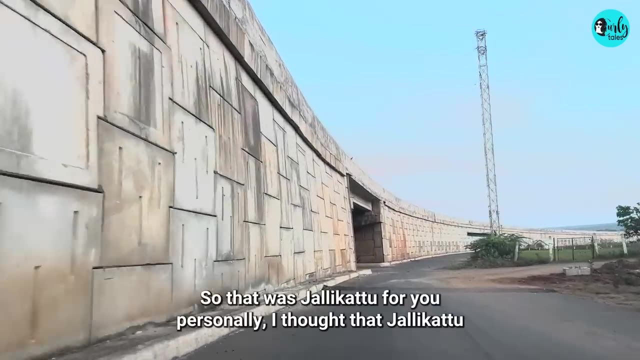 stay, accommodation, food and so much more. And the best part is, this is available across Marriotts in the whole world. So grab your friends and sign up for the Loyalty Programme. So that was Jallikattu for you. 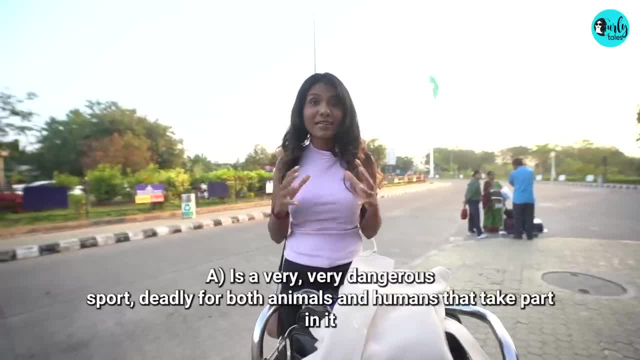 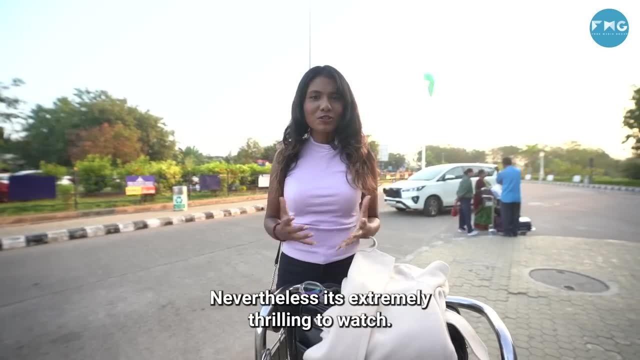 Personally, I thought that Jallikattu-e is a very, very dangerous spot, deadly for both animals and humans that take part in it. Navratilis is extremely thrilling to watch. Is it cruelty? Well, from what I've seen, the people of Tamil Nadu really worship their bulls from. 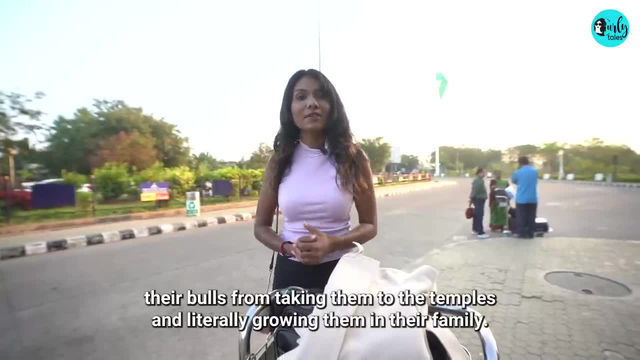